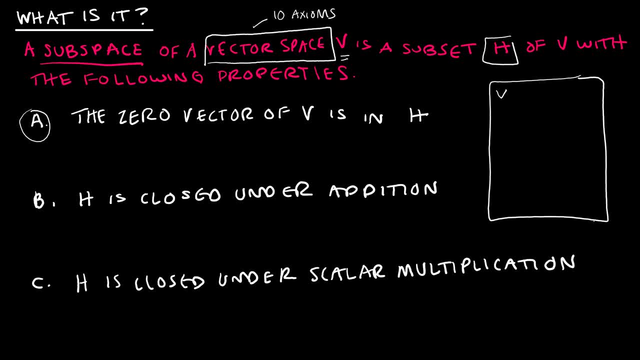 So this is just my random vector space containing whatever I want it to contain. really, Within that small or equal to V is H, which is a subspace, And so notice, I've drawn it inside V, which means it contains values that are in V. So let's say 312 was not in V, then it's also not in H, So it. 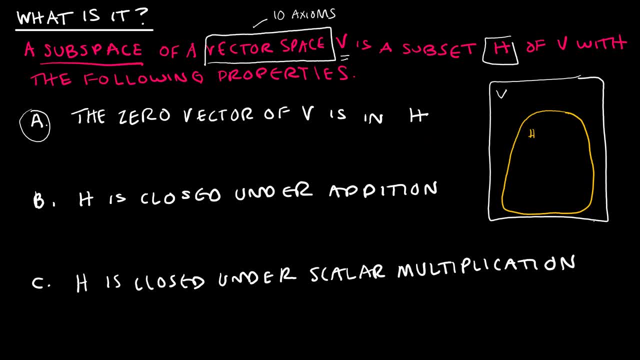 has to be something that's already in V in order for it to be in H. It's a subset, So the first one is the zero vector. So what I'm going to do is I'm going to take the zero vector and I'm going 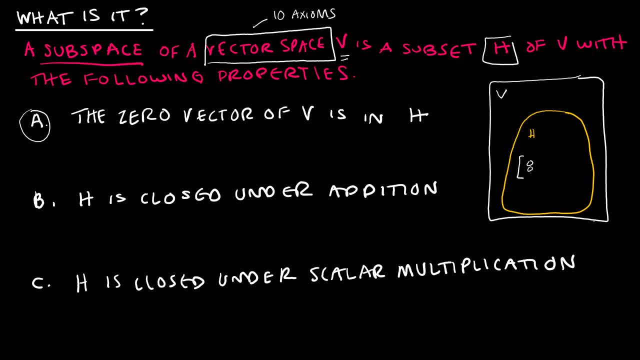 to put it in H. So what I'm saying is, let's say: these are, you know, R3 vectors: The zero vector, 0, 0, 0, must be in H in order for it to be a subspace. Also, we need to know, and again: 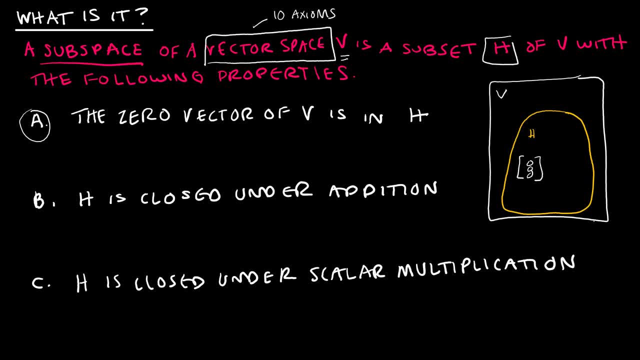 this. we would say that let me change colors here- that zero belongs to H And again zero means the zero vector H is closed. under addition says that if you've got, say, vector U and vector V that are in H, so U and apparently U again. 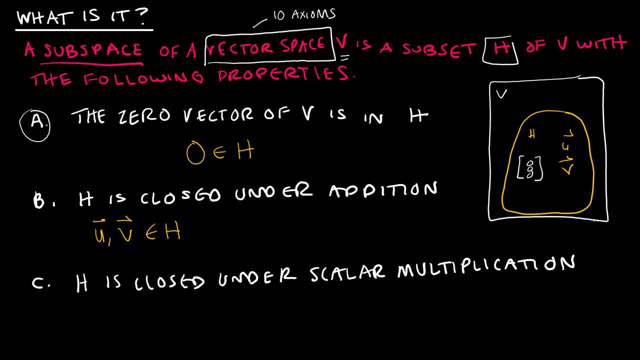 U and V that are in H, then if I take U plus V, that must also be in H. So U plus V must also be in H. Also we need to say that H is closed under scalar multiplication. So if U is in H, then C, U is in. 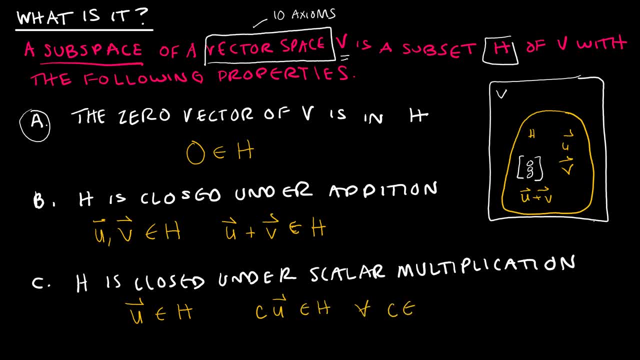 H for all C's. that are real numbers, So I should be able to take my vector U times anything, and that should also. that resulting vector that has been multiplied by the scalar multiplication should also be within H. So those are the three properties. Now keep in mind that V has already. 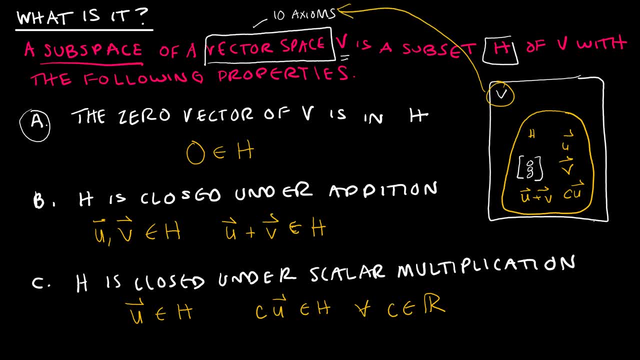 met these 10 axioms. So for H we really just need to check that these still hold true for that smaller, typically smaller subset. I would also point out that every subspace is then a vector space. So once we meet that vector space, we're going to have a vector space. So once we meet, 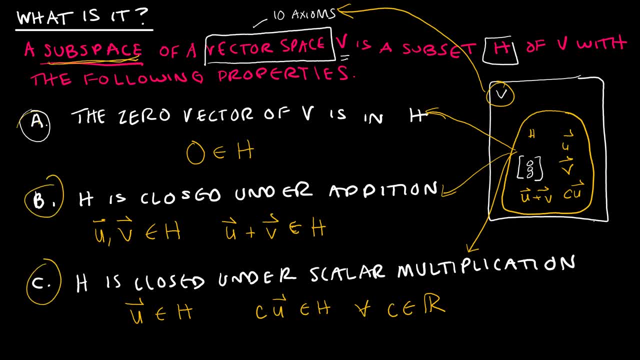 that vector space, we're going to have a vector space. So once we meet that vector space, we're going to have a vector space. So once I have this requirement, using these three properties, those subspaces are all vector spaces. So we don't have to then check the ten axioms. we 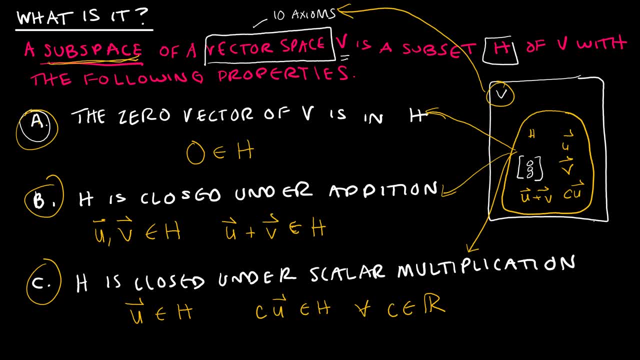 only have to check these three. We can also say that every vector space is a subspace, and that means it's a subspace of itself. So, as I said, H could be the exact same size as V, or it could be that that vector space is a subspace of some larger vector space. 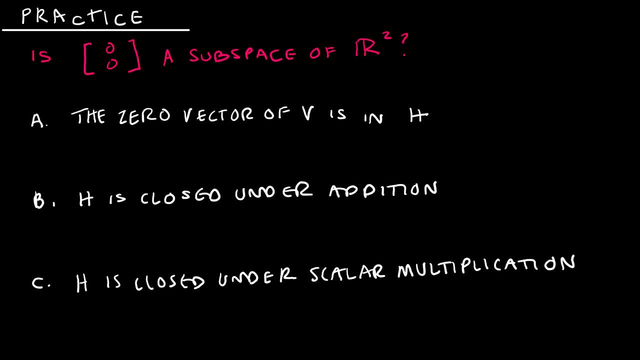 Here's a fairly straightforward practice question for us to look at together. So notice I have, which is the zero vector, And I'm asking: is this zero vector a subspace of R2?? So I could have just as easily said is the zero vector and not specified that it was. 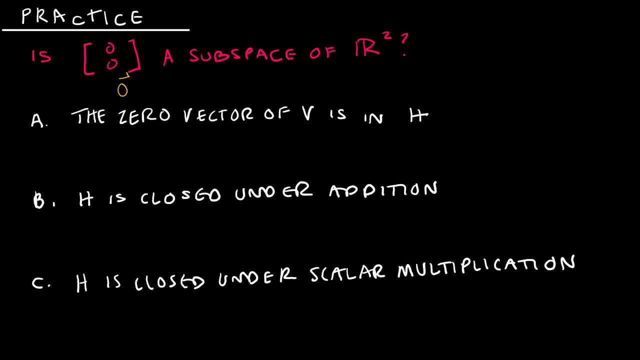 two, two rows, a subspace of Rn, And my solution here would be the same. So, essentially, I'm saying that H is only the zero vector. That's it. So the zero vector of V is an H. Well, yes, because the zero vector is H, And so, obviously, 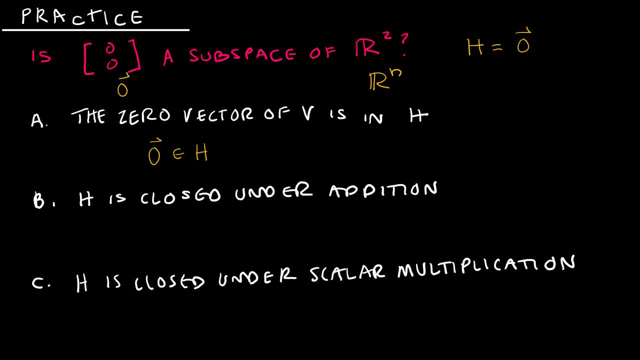 that is an H. H is closed under addition. Well, if I take the zero vector plus the zero vector, I get the zero vector, which is an H, And therefore it is closed. So closed under multiplication, I'm sorry. addition simply means if I take any two values. 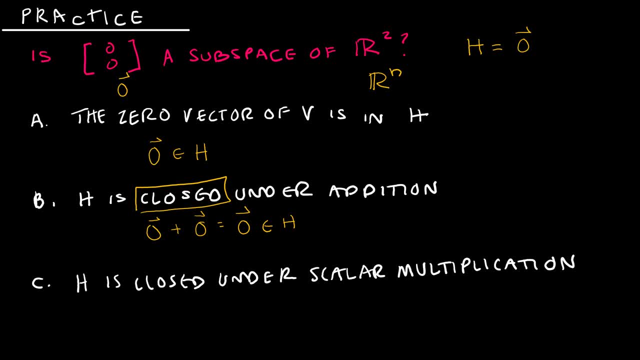 within H and add them together, that that new value is in H as well, And that, of course, is true. H is closed under scalar multiplication. Again, it's saying if I take anything in H and multiply it by a scalar, that result is: 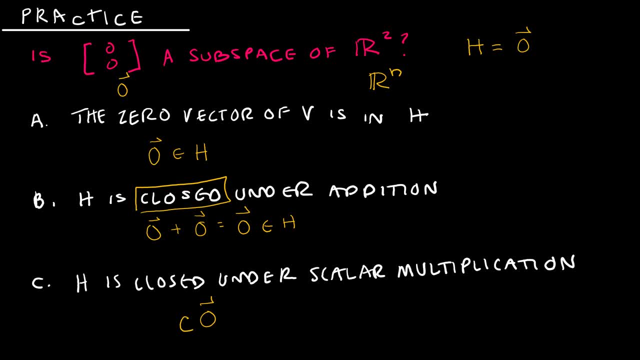 in H. So again, if I take C, any C times the zero vector, I will get the zero vector, And we already know the zero vector. We already know that the zero vector is in H. Therefore, yes, this is true not only for 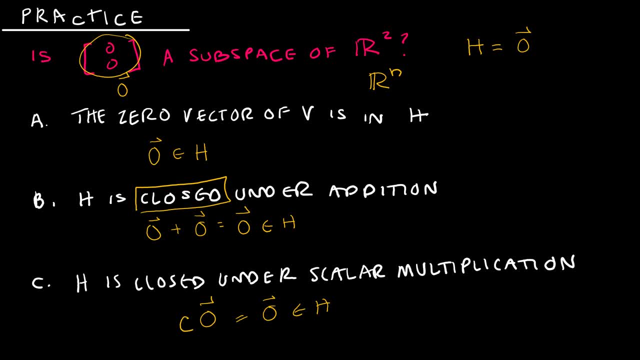 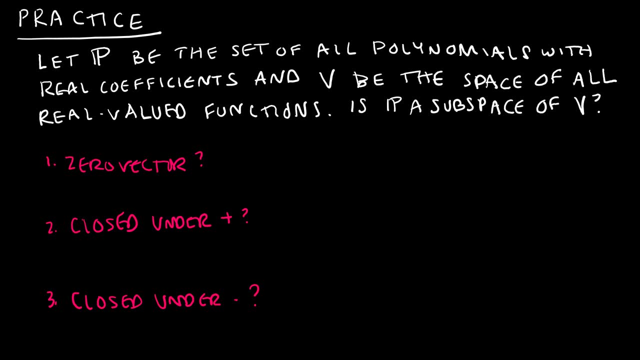 this particular vector, 0, 0, the zero vector for R2, but really for any Rn. Here's another question for us to look at. Let's let P be the set of all polynomials with real coefficients, So real number coefficients. 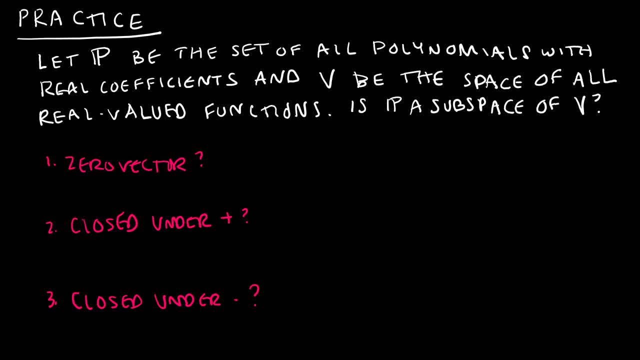 And V be the space of all real valued functions. So they're telling me here That V is the space of real valued functions, meaning V is does meet all of those 10 axioms. I don't have to check the axioms for V, But V is the space of all real valued functions. 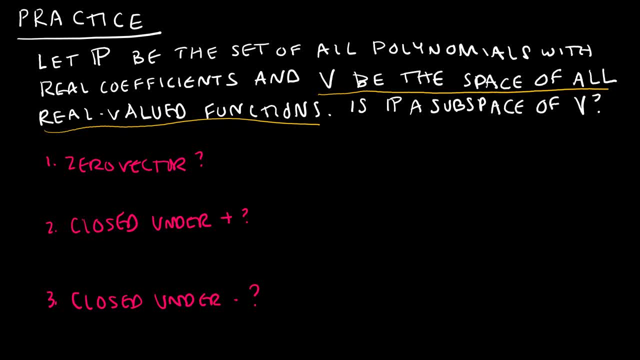 So not just polynomials but any real valued function. The question is: is P, which is the set of all polynomials with real coefficients, is that a subspace of V? So I've just sort of jotted down the basics of those three. 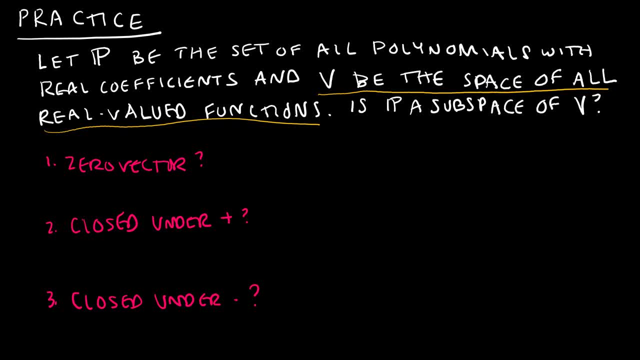 And I'm going to check out the other properties that we need to check. So I wrote zero vector, But here essentially I'm saying zero polynomial. Is that in the set? Well, obviously it would make sense that I could have the polynomial 0.. 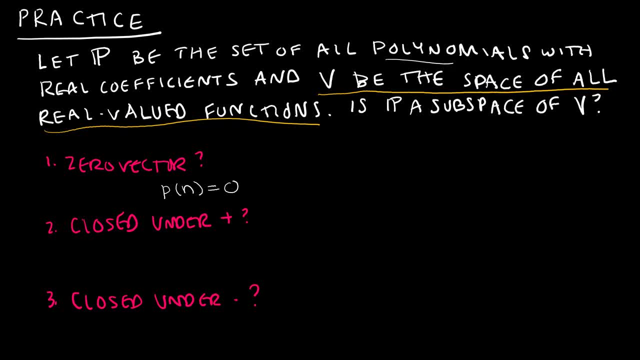 That would be the set. It would be in the set of all polynomials with real coefficients, And so, yes, that is in the subspace Closed under addition. So we've kind of talked about this already. If I had A of t which was a0 plus a1, t1,, t to the first plus a2, t squared, et cetera, 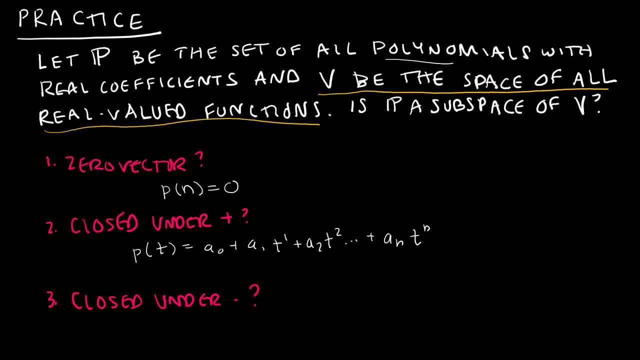 And I won't say et cetera, et cetera, because someone had an issue with that and left me a comment about it. Thanks so much. So this would be b sub 0.. And then whoops, b sub 0.. 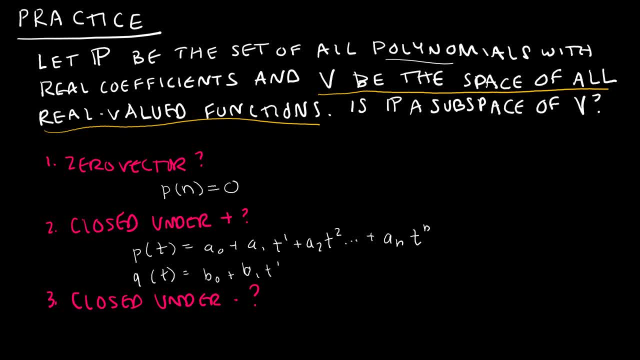 Nope, b1.. t to the first. We get the idea. Oh, I keep switching a's and b's, b and t to the n, So closed. under addition, If I added these together, we talked about how this would look. 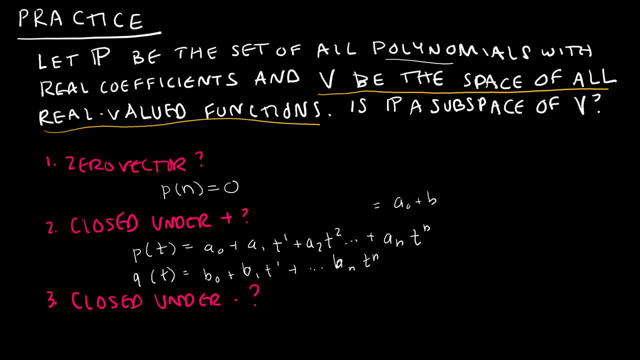 I would have a0 plus b sub 0 plus a sub 1 plus b sub 1, t to the first, et cetera, And would that then be A polynomial with a real coefficient? Yes, it would, Same thing with multiplication. 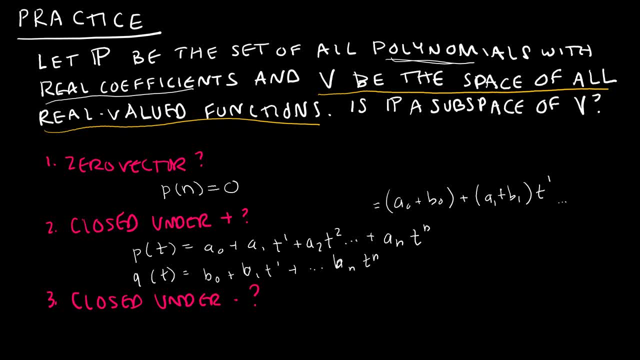 If I were multiplying these instead. it's going to look like this without the addition sign in between, And it's going to be a little more involved than this because obviously it would involve some distributive property. But it's very clear that if I took a0 times b sub 0 and times b sub 1, et cetera, that all of these would be equal. 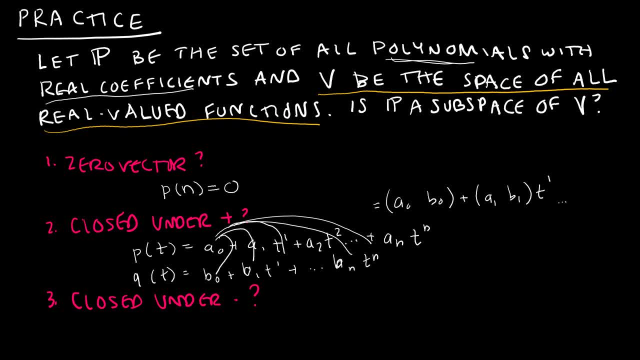 All of my values will in fact have real coefficients And there would be some combining of like terms. But yes, my resulting equation would in fact be a polynomial with real coefficients. So I didn't really write down anything for that, but hopefully that made sense to you. 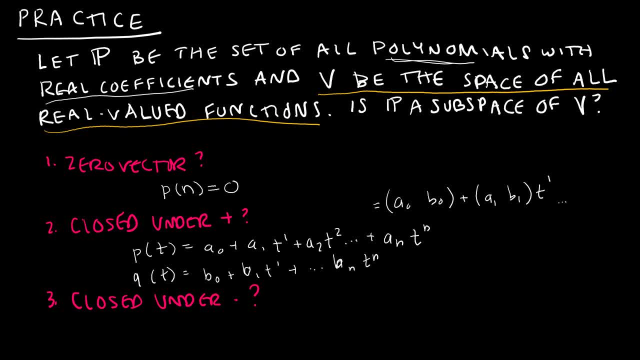 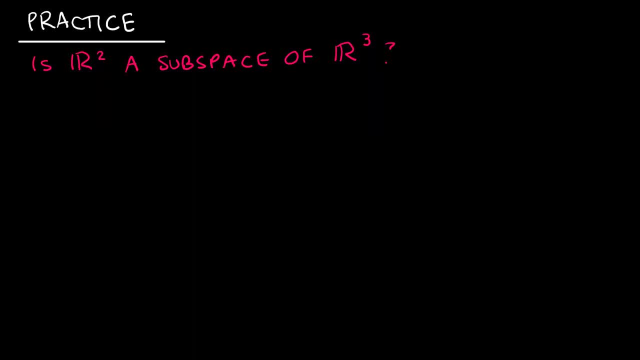 Yes, the set of p would be a subspace to all real valued functions. How about this one? Is r2 a subspace of r3?? So you might be thinking: well sure, r2 is smaller than r3 because 2 is smaller than 3.. 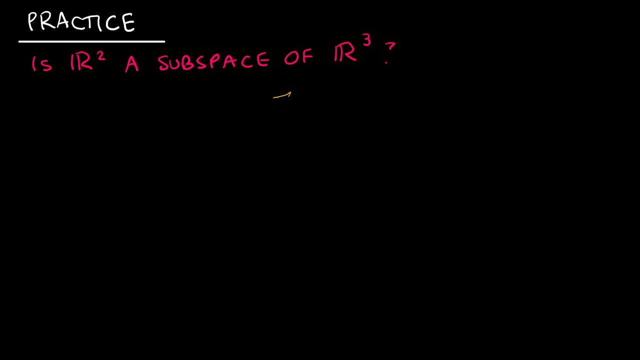 But remember our cute little picture that we drew before. If this is r3, which would of course be any vector with three entries, is it possible that r2 is inscribed The side of there, r2 being vectors with two entries? 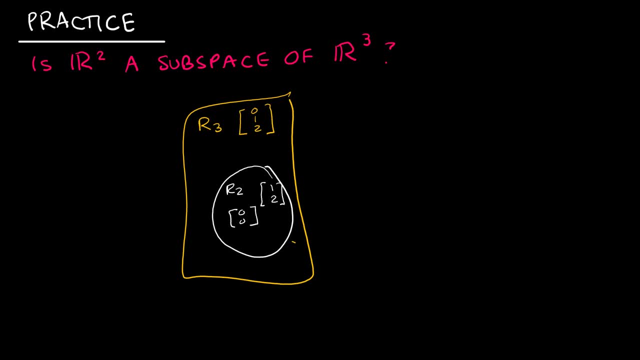 Does that even meet the initial requirement? before I start checking properties, Is it in fact a subset? No, it is not, because r2 has two values and r3 has three values, And so r2 is not a subset. Now if I wanted to take r2 and say r2 has 0,, 0, and I'm going to add a 0 as the third entry, 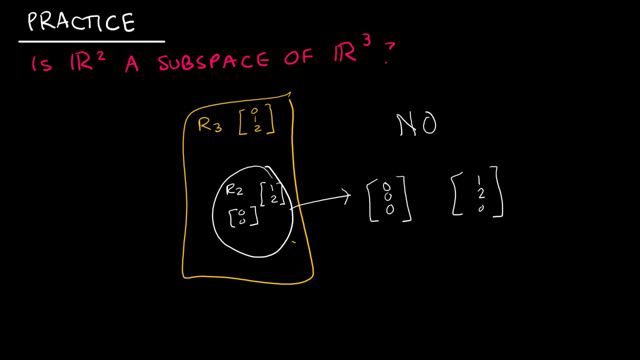 and r2 has 1.. And I'm going to add 0 as a third entry. These certainly do belong in r3 as well as r2.. Sorry, these certainly do belong in r3, but then they would no longer be in r2.. 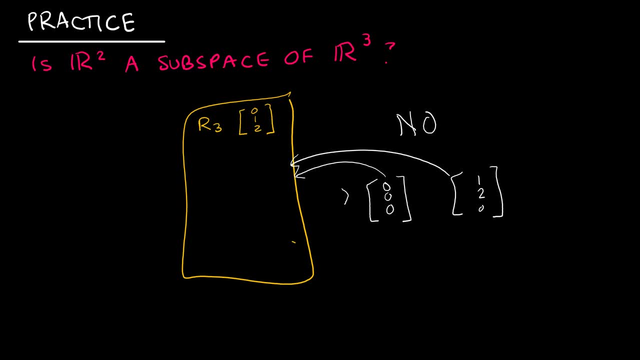 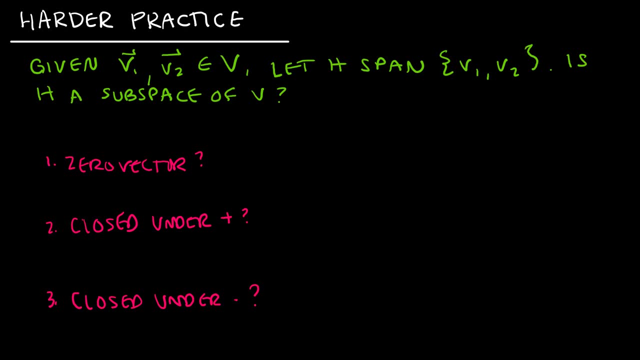 So r2 cannot be a subspace of r3, again because it doesn't fit even the same pattern. Let's do a harder practice question. If I'm given that v1 and v2 are vectors and h spans v1, v2,, is h a subspace of v? 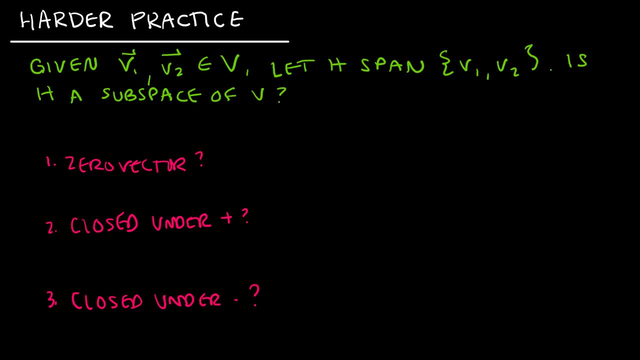 So, before we go about checking our properties, just recall that this is telling me that I should be able to write everything as a scalar whoops: a scalar times the vector plus a scalar times the vector, And that's what it's going to look like to be an h. 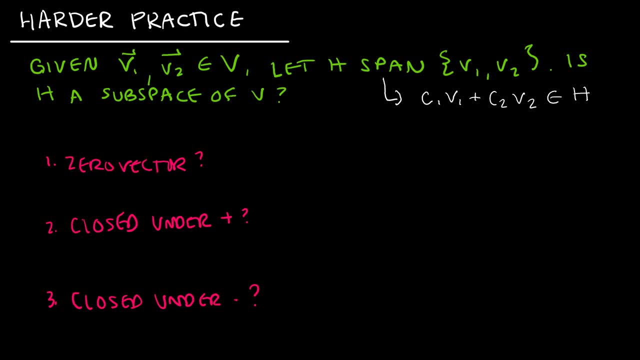 I can write it. I can write it as a linear combination of those vectors. So is the 0 vector in h? That's what they're asking- Is the 0 vector in h? Well, I can certainly write 0 v1 plus 0 v2,. 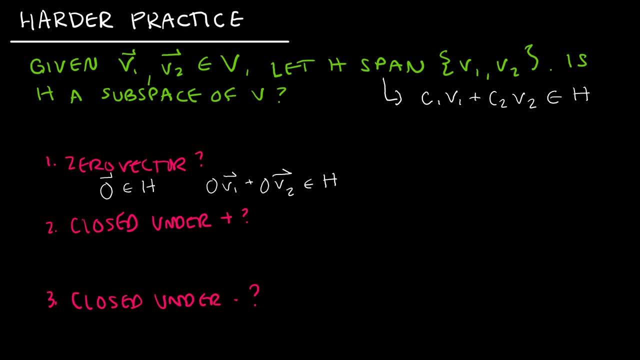 and that would in fact be the 0 vector and it would be in h. So yes, Is it closed under addition, Meaning if I have u and v that belong to h, so they already have to belong to h. the question is when I add them together. 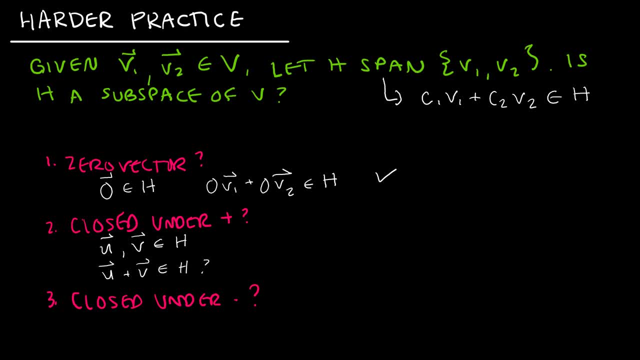 is the result also in h. So that's what I need to check And I want to caution you here, because I see this a lot on homework and even quizzes and tests, where someone will tell me that vector u is 2v1 plus 3v2,. 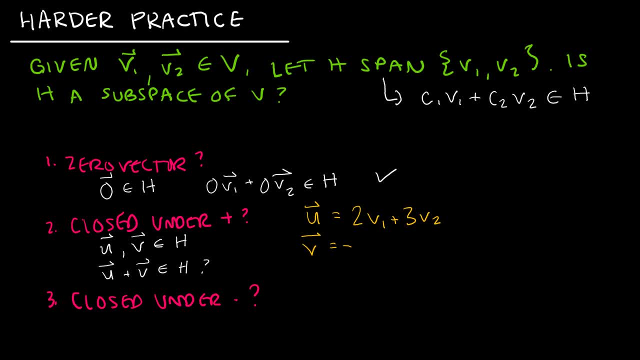 and that vector v is negative: 4v1 plus v2.. Well, that's well and good, except these are specific values and in order for us to prove anything, we need to use obviously generalized values. So instead of plugging numbers in here, 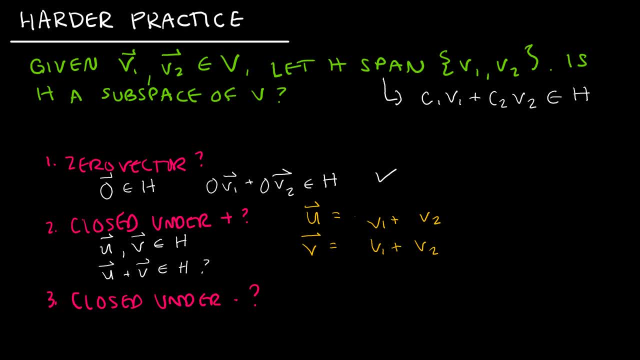 I'm going to say say s1v1 and s2v2, and t1v1 and t2v2.. Because now it's not a specific number, because, remember, with specific values I would have to check all of the specific values. 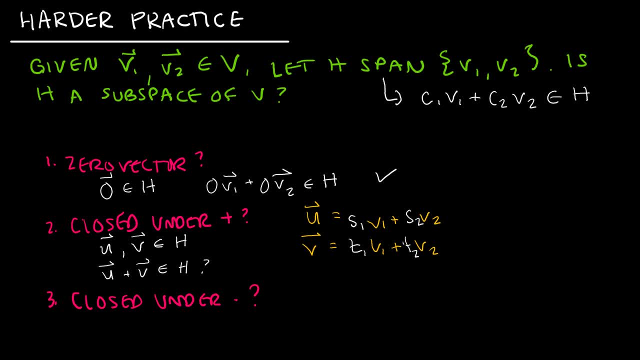 which is impossible because there's an infinite amount of specific values. So use these generalized values, then show that with these generalized values that my result would in fact be in h. So let's take u plus v By combining like terms. 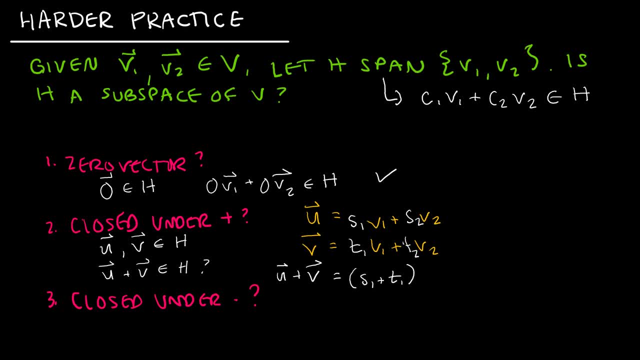 I would have s1 plus t1, v1, plus s2 plus t2, v2.. Does that belong in h? Yes, it does. Again, whoops, don't cross it out. It can be written as a linear combination of vectors v1, v2.. 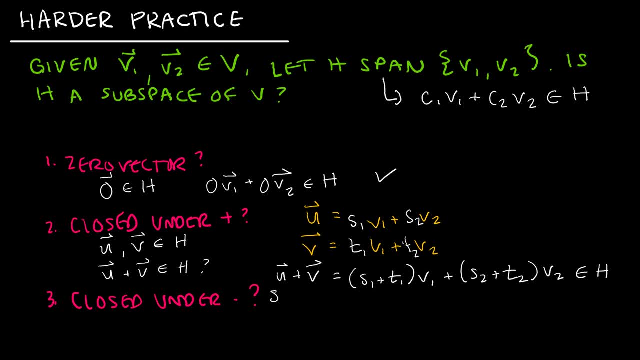 Lastly, let's look at closed under multiplication And again recall: this is scalar multiplication. I didn't specify that when I wrote down closed under multiplication. but that's what we're talking about. We're saying c? u- is that in h? 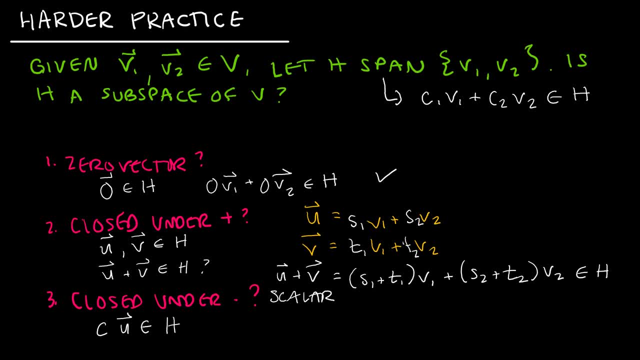 Again, assuming that u is in h, as I said before, then is cu in h, And so let's take a look at what cu would look like. That would be c times s1, v1, plus c times s2, v2.. 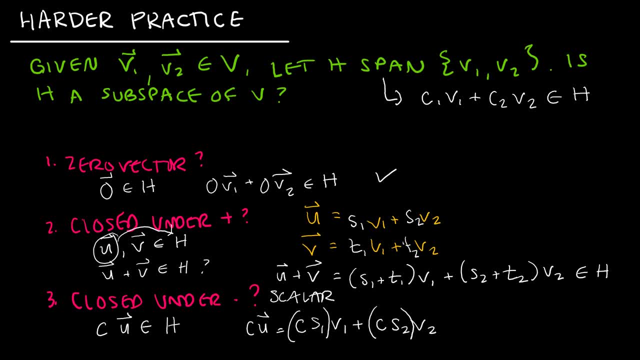 And again, just by using some parentheses here it's very clear. it's very clear that, yes, this belongs in h. So we've sort of generalized it for v1, v2, but no matter how many vectors we have in a vector space, 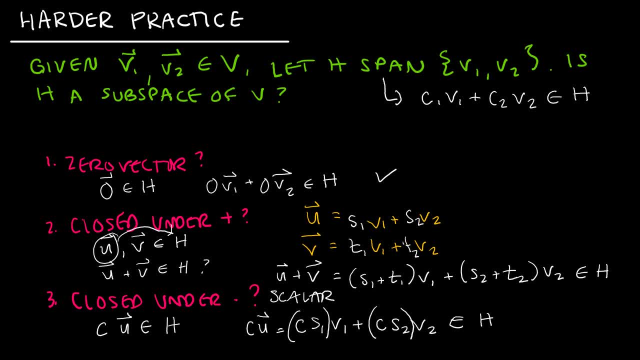 then it will always be true that the span of those vectors is a subspace of v. That's theorem one in your textbook. I'm not going to write it down, But again, you could prove it for any number of vectors the way that we did here for just two vectors. 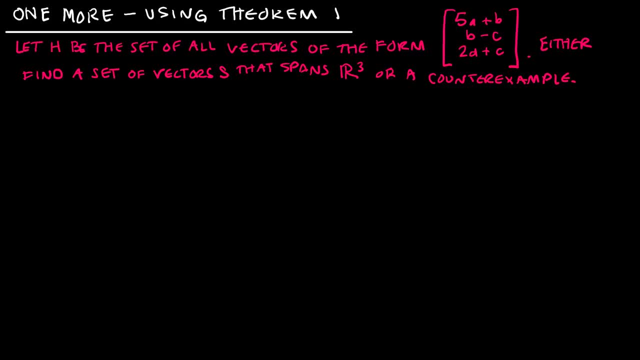 Let's do a question now using theorem one. As you recall, we just talked about theorem one that says: if we have vectors in the vector space v, then the span of those vectors is a subspace of v. So here we are, asked to let h be the set of all vectors. 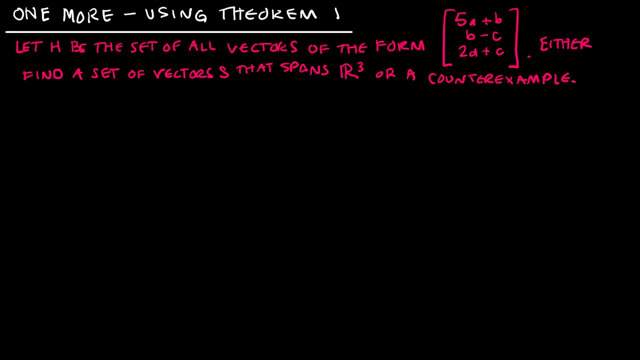 in the form 5a plus b, b minus c, 2a plus c. And then it says: either find a set of vectors that spans R3 or a counterexample. So they're asking us to essentially find v1,, v2,, v3,. 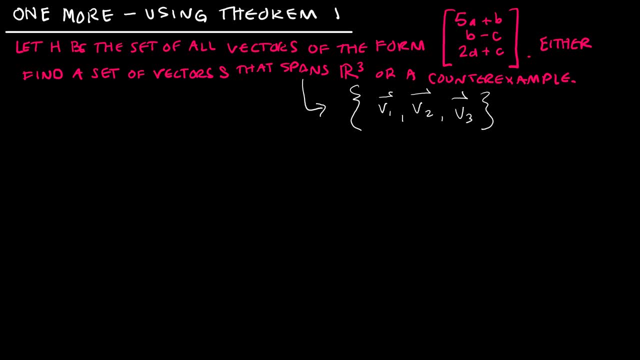 or show that that's not a possibility. And this is actually far more straightforward than it might appear. What I'm going to do is I'm going to say, if I've got my 5a plus b, b minus c, 2a plus c. 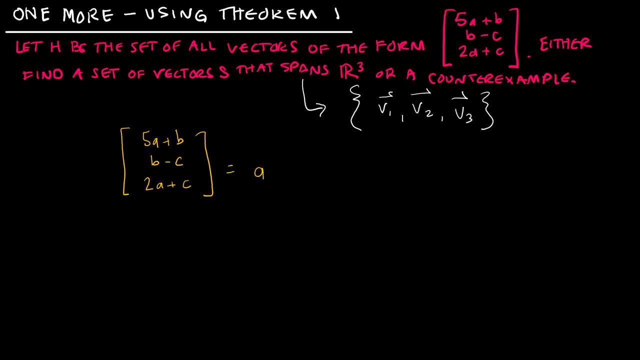 then can't I write this as a times: v1 plus b, v2 plus c, v3,, which would show that it's a set of vectors that spans R3.. So essentially what I'm saying is, if I'm able to find that v1, v2, v3,. 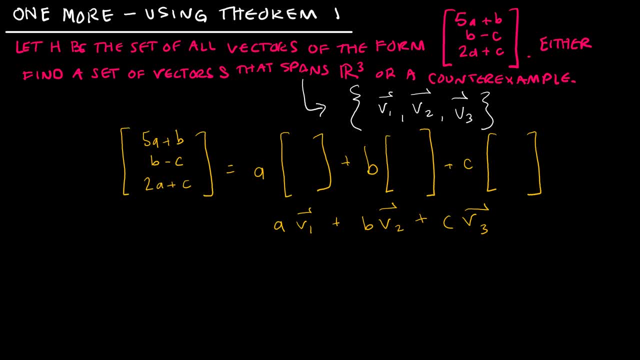 then I've done exactly what they asked. I've found the set of vectors, which would be v1, v2, v3, that spans R3.. So how am I going to do this? Again, very straightforward. This is 5a plus b, so that's 5a plus 1b plus 0c. 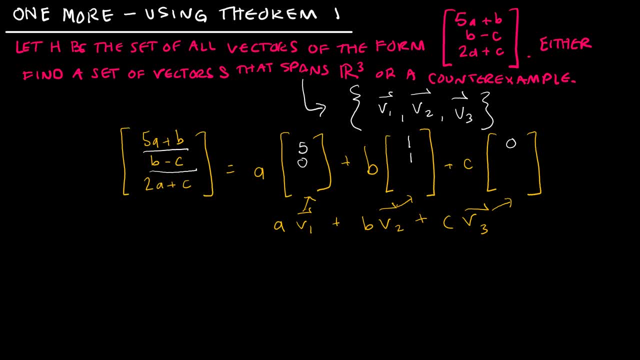 This is b minus c, so 0a, 1b negative 1c, and then 2a plus c, so that's plus 0b plus 1c. Okay Voila, I've found the set of vectors S. 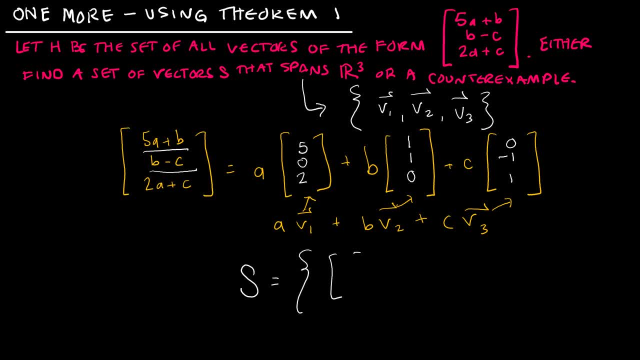 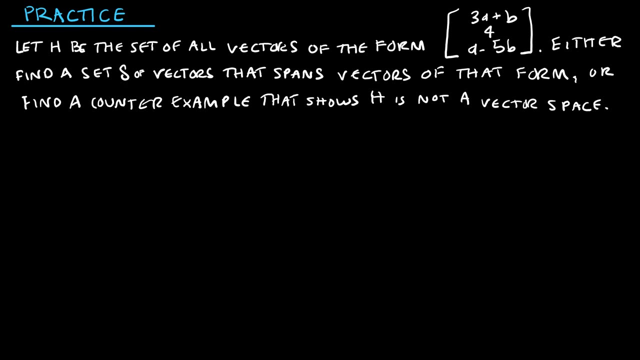 to be 5, 0,, 2, 1, 1, 0, 0, negative: 1, 1.. Last one for you to try on your own Press pause. Try this question when you are ready. 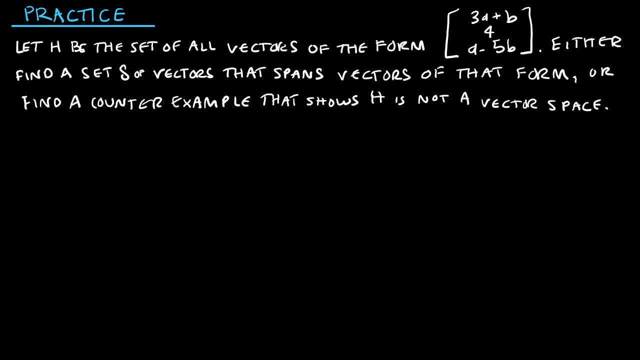 Press play to see how you did So likely. you started about this in the same way. we did the last one and we said 3a plus b, 4a minus 5b. and then you might have said, oh well, this guy looks a little different. 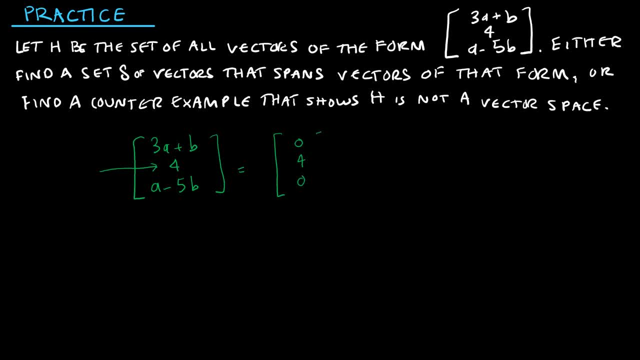 so maybe I'm just going to have a 0,, 4,, 0 as a constant and then a times some vector and b times some vector. but this actually is not the case. So it says: either give vectors that span, vectors of that form. 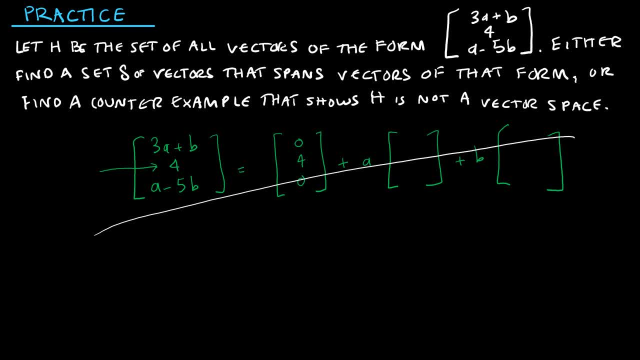 or find a counterexample. So I can show a counterexample showing that in fact the zero vector does not belong to H and therefore it cannot be a vector space, and the reason for that is again because of that 4.. 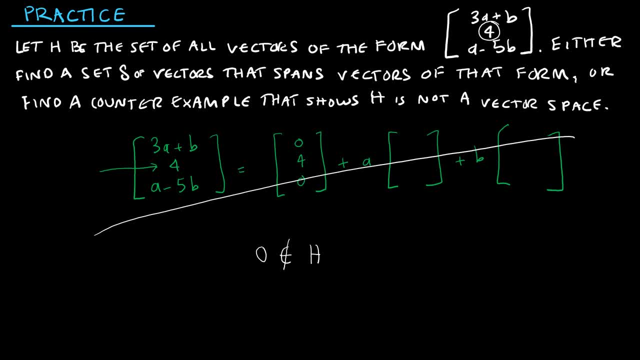 So in this case I don't need to do any other work except to show that H is not a vector space. That's it. 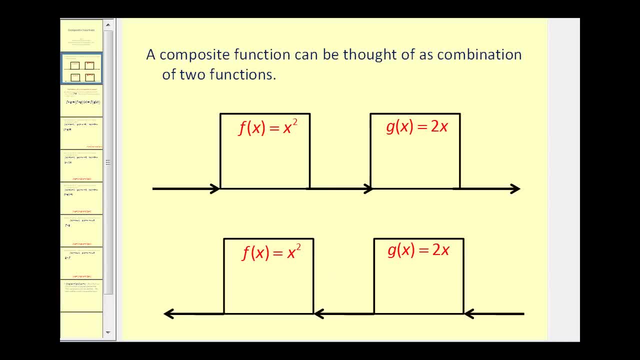 Welcome to a video on composite functions. A composite function can be thought of as a combination of two functions. One way to illustrate this would be to use a conveyor belt where we have an initial input, let's say 3.. One way to illustrate this would be to use a conveyor belt where we have an initial. 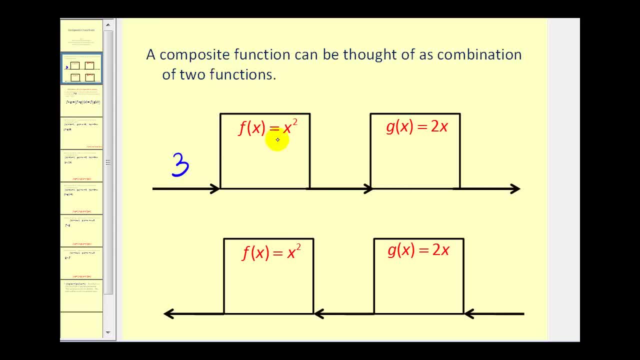 input, let's say 3, and it becomes the input into f, where f squares its input and produces an output of 9, and this output becomes the input into g. So we multiply 2 times 9 and the final output of this composite function would be 18.. 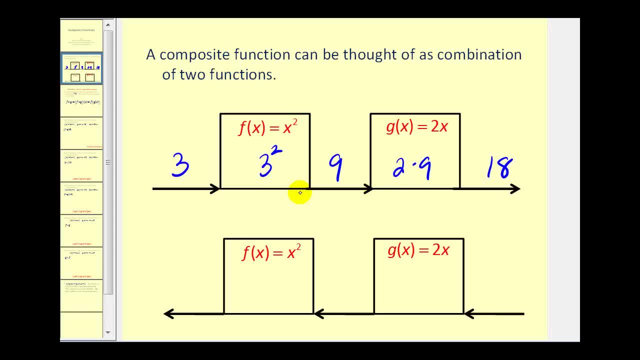 Now, the order in which we evaluate a composite function is extremely important. So, for example, if we have the same functions but now we reverse the order and we start with the same input of 3, function g would multiply that by 2, producing an output of 6.. 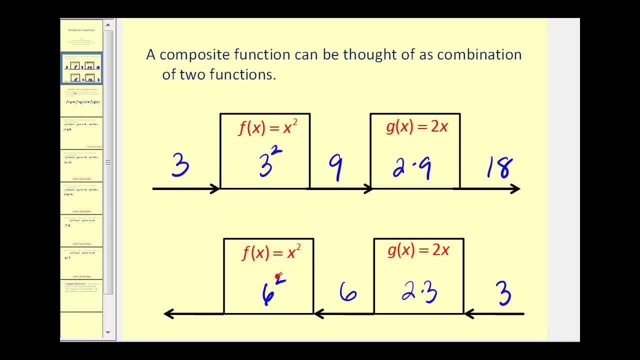 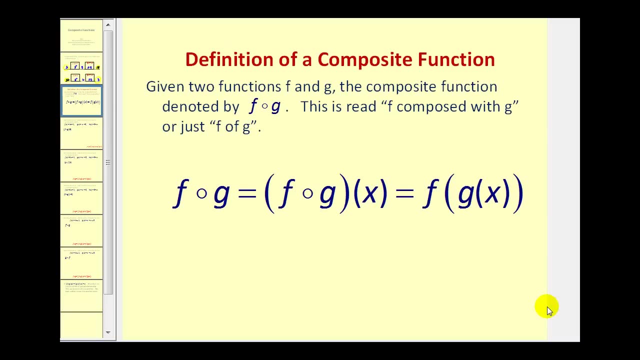 Which becomes the input into f, and 6 squared would be 36.. So notice, if we change the order in which we compose functions, the outputs in most cases will be quite different, Even though our inputs may be the same. The formal definition of a composite function states: given two functions- f and g- the